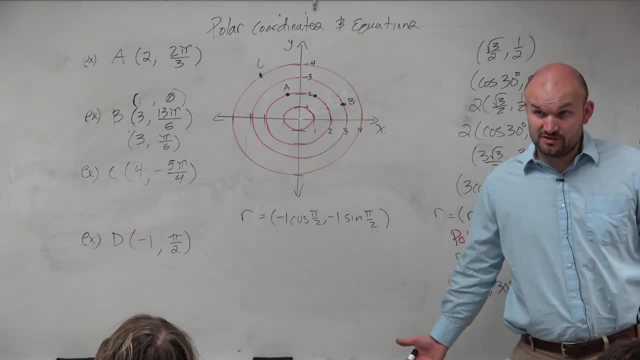 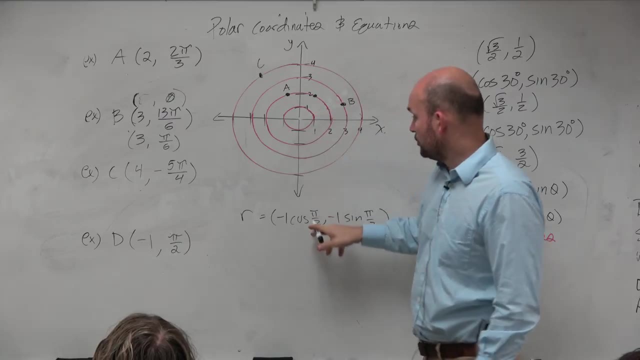 Would you guys agree? that's the rectangular form of that. Now let's see. Think about this rectangular form. Well, cosine of pi halves. pi halves is, we look at the unit circle, pi halves is 90 degrees right. So the cosine of pi halves is 0, 0, comma sine of pi halves is: 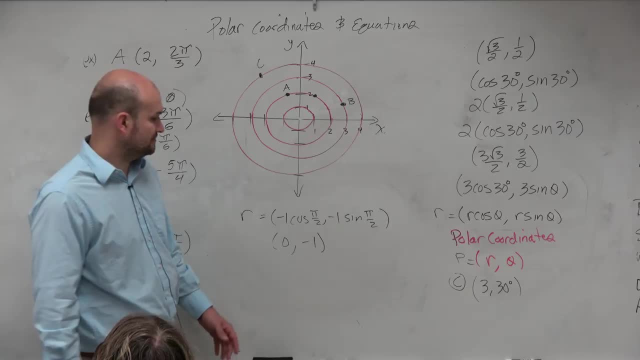 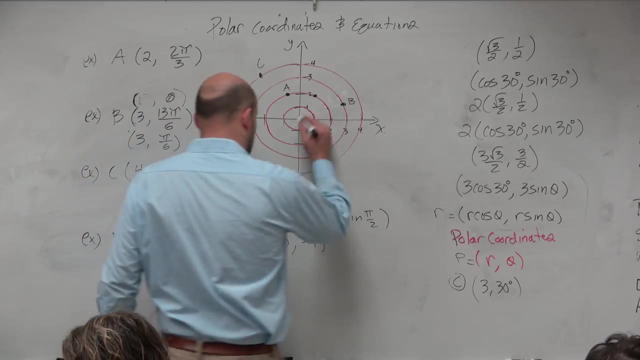 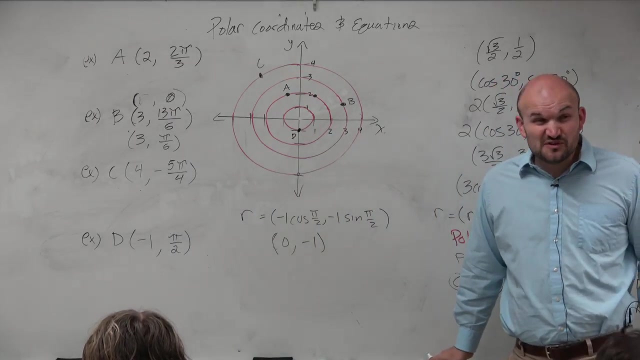 1. So that becomes a negative 1. I'll give you your test in a second. Just have a seat. So the point for D is all the way down here. But that gets confusing, doesn't it? Because if you were to think about this as 1 half, 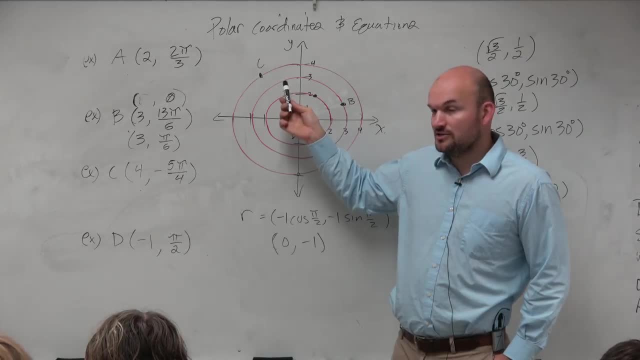 you would just think of: well, well, Mr McLogan, 1 half's up there, So why is it like down here, Right? Isn't that confusing? Yeah, Yeah, No, it's not confusing. Well, it confuses a lot of people. 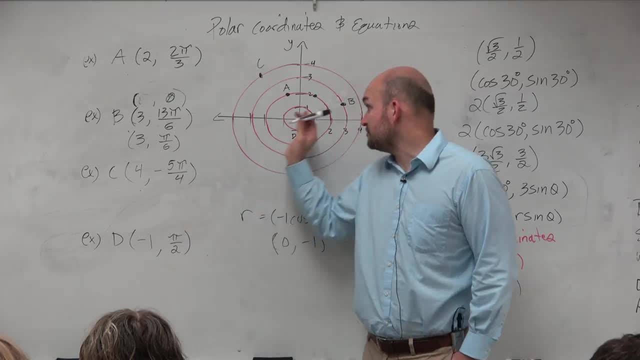 especially when you graph, like if you forget about the negative. If you were just to graph pi halves, you would say it's up here, But what happens? is this negative? you guys got to think that's like a scalar multiple, right. 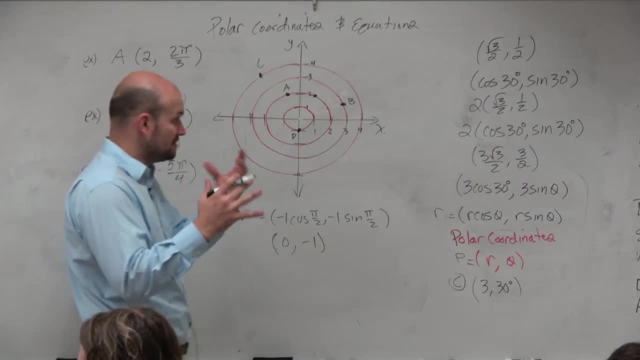 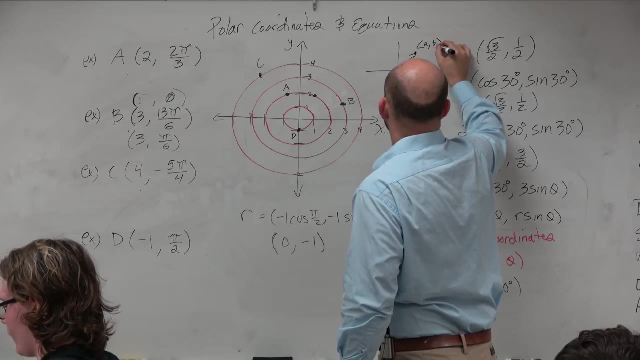 And again the way that I can visually, if we go back to remember how we're connecting so many things with vectors, If you guys think of a vector, let's say this vector here is ab. What happens when I multiply that vector times a negative? 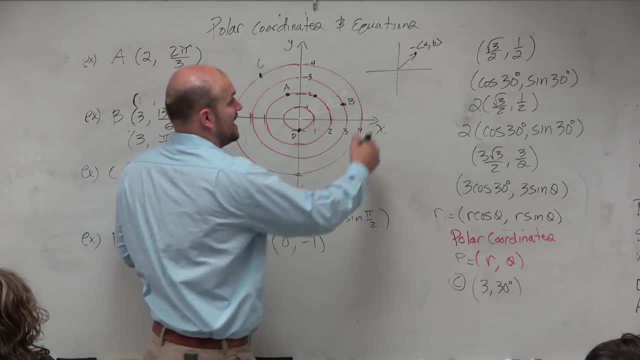 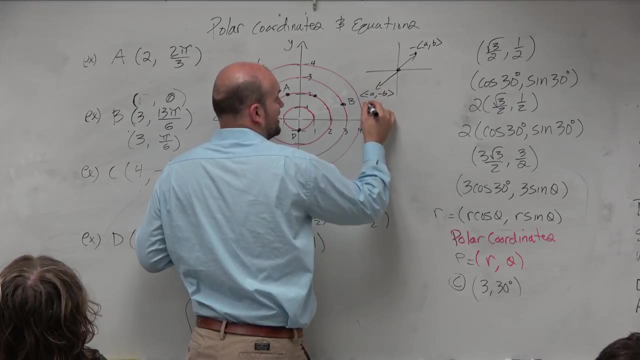 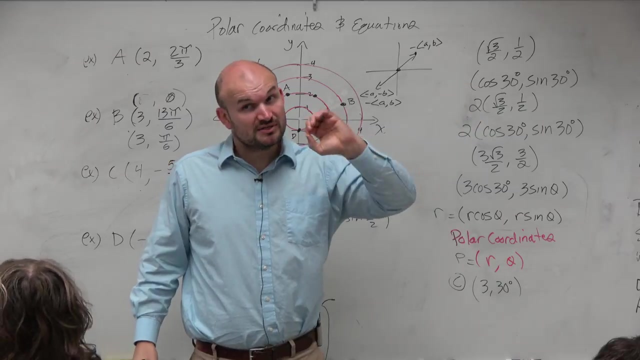 by a scalar multiple of a negative. Where did that graph go? Well, this now becomes Negative a comma, negative b right When I do negative ab right, Because you distribute that negative to both in one of those terms. So what's important about this is because a lot of students 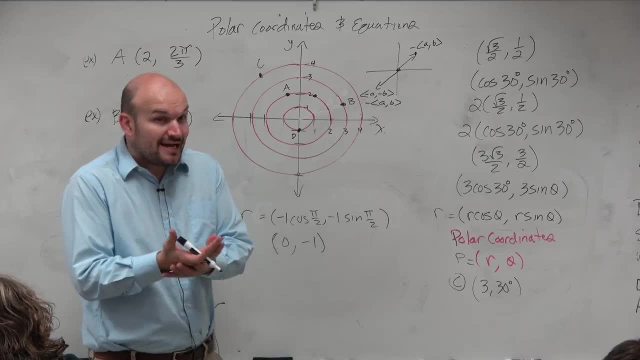 will look at this and say, Mr McLogan, well, radius cannot be negative 1.. Well, yeah, your radius is not negative 1.. The radius is still a value of 1.. But you got to think this is representing. 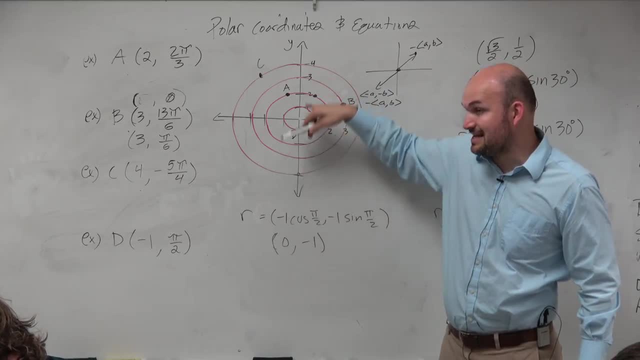 this is like a direction. This is taking you this distance. It's not taking you to. the distance is going to get 1.. The distance is going to get 1.. It's still 1.. But now what this is doing is it's. 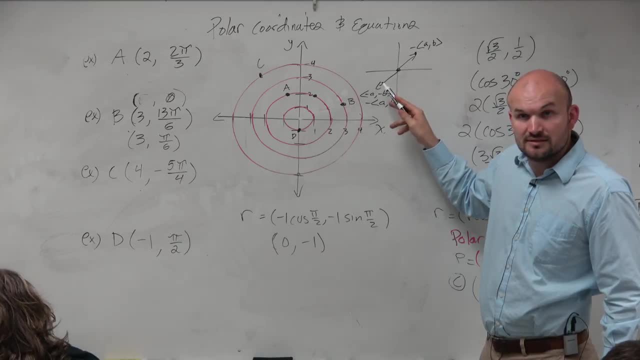 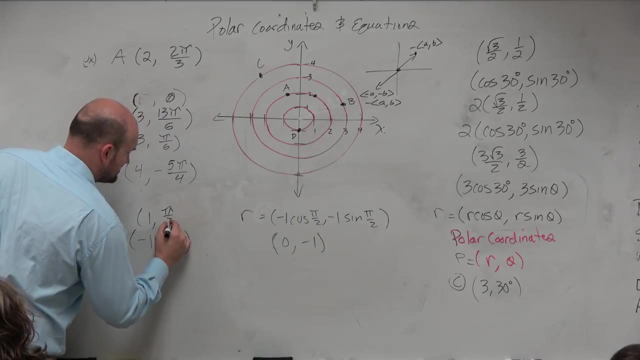 kind of changing the direction, like we did with vectors. right, So we're changing the direction. So, when this is negative, what that's doing is it's taking 1 comma pi halves, which would be right here. It's taking 1 comma pi halves and it's